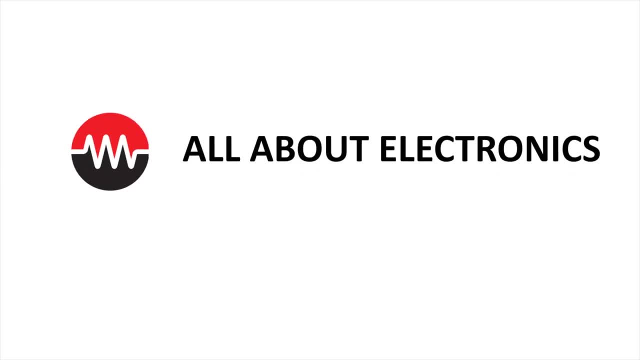 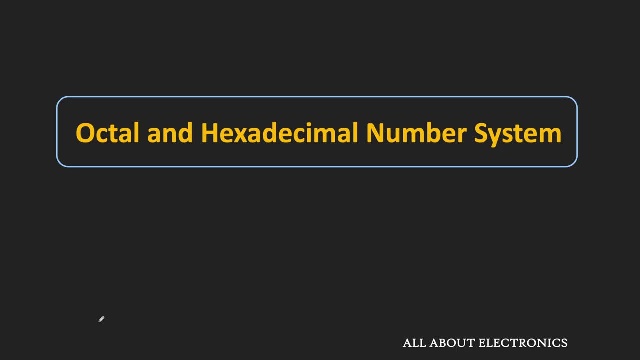 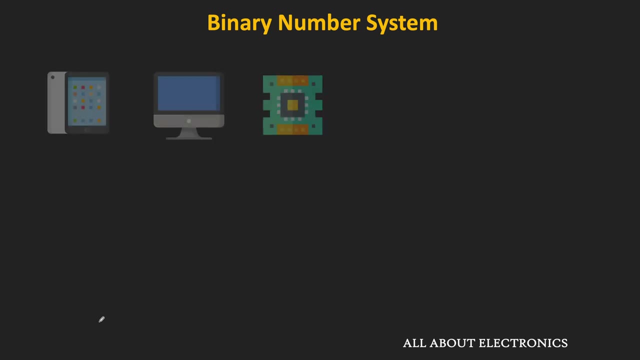 Hey friends, welcome to the YouTube channel ALL ABOUT ELECTRONICS. So in this video we will learn about the octal and the hexadecimal number systems. So, as you know, the computers and the digital circuits works on the binary number system, which consists of only 1s and 0s. 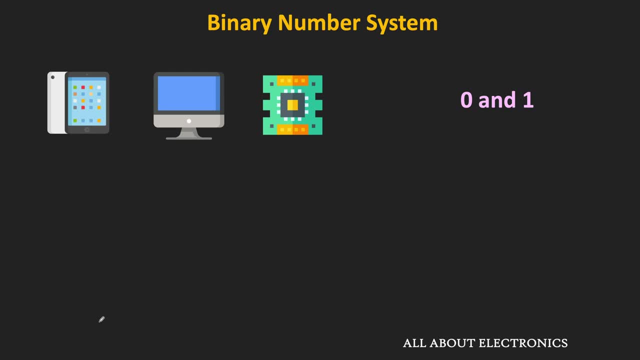 Now, these binary numbers typically requires 3 to 4 times more digits than the decimal numbers, And therefore the computer works on very large binary numbers And in fact, nowadays even a 64-bit binary numbers are also very common, So these numbers could be some numerical data, or it could be some memory location, or even 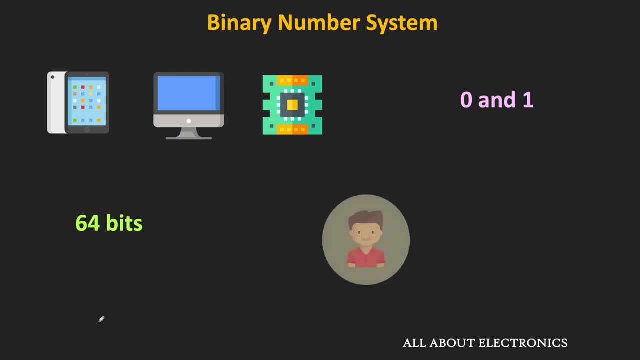 some instruction code. So whenever a human operator or the user wants to interact with the computer, then dealing with such large binary number becomes very difficult, And in such case this octal and the hexadecimal number system is very useful. So now, if you see this octal number system, then it consists of total 8 symbols. 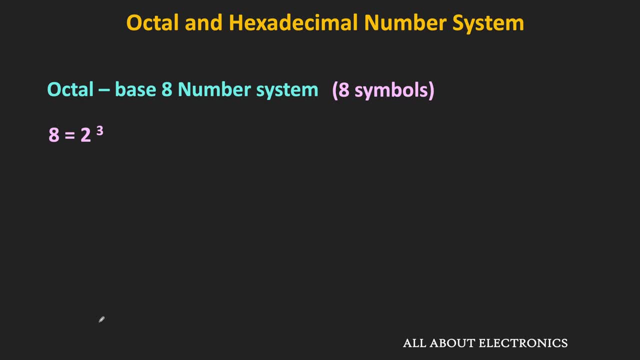 And, as you know, these 8 can be represented as 2 to the power 3. Meaning that every 3 bits of binary numbers can be represented just by 1 octal digit. So if we have a 12 bits of binary numbers, then in the octal number system it can be: 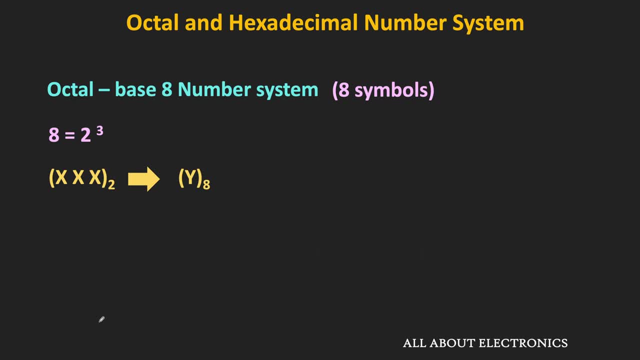 represented just by only 4 octal digits. It can also be represented by multiple octal numbers. On the other hand, this hexadecimal number system is a base 16 number system which consists of total 16 symbols. So, as you know, this 16 is equal to 2 to the power 4.. 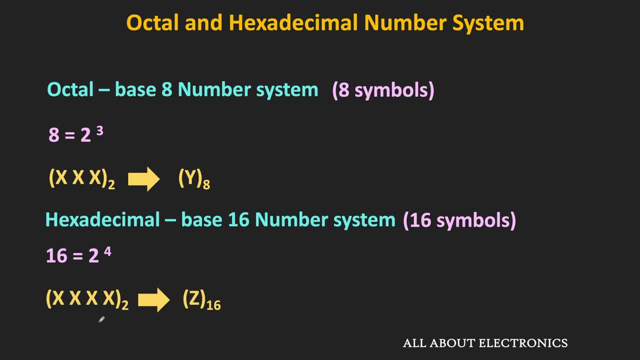 That means every 4 bit of binary number can be represented just by only one hexadecimal digit. So if we have a 16-bit binary number, then in the hexadecimal number system it can be represented just by only 4 hex digits. That means by using this octal or the hexadecimal number system- this interacting with the computers- 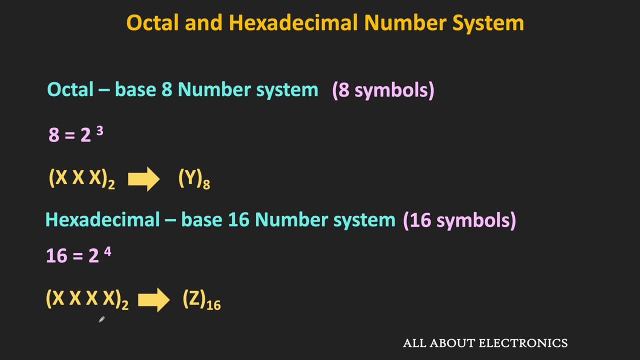 becomes much easier for the user or the operator. So throughout this video we will learn the following topics, But first let's start with the octal number system. So, as I said, this octal number system is the base 8 number system and it consists: 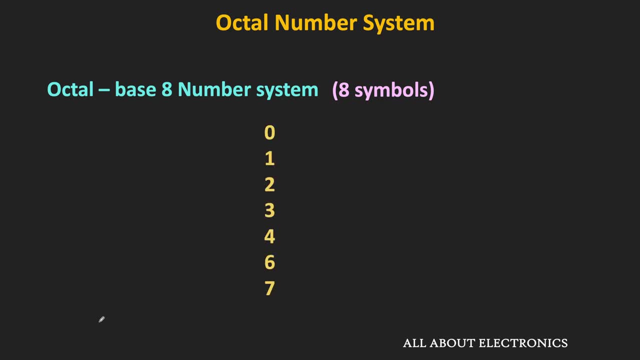 of total 8 symbols. So here is the list of all 8 symbols. Now, if we want to count in this octal number system, then it is very important to know that the number is very similar to the decimal number system. That means once we use all the symbols for the counting in that particular number system, 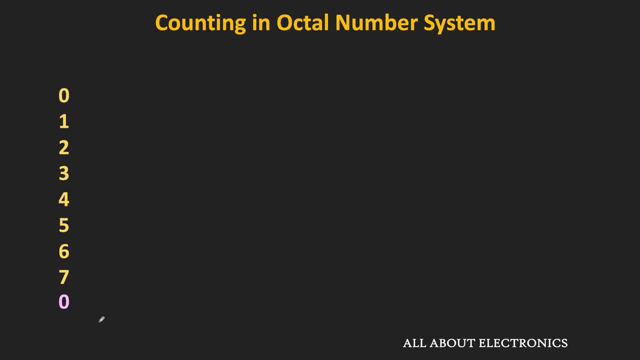 then we will reset that column to the 0, and we will increment the next column by 1.. That means the next number will be equal to 10.. So once again, the counting will go up to 17.. So, once again, since we have used all the numbers in that number system, so we will. 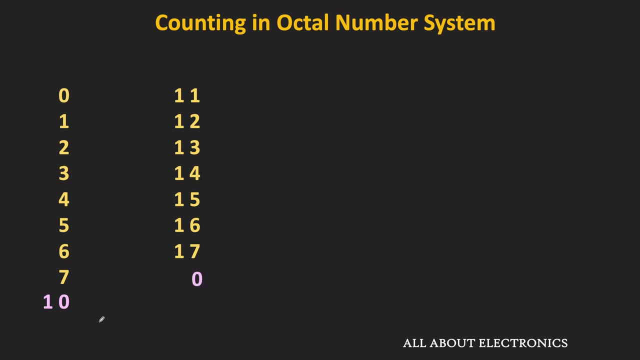 reset the rightmost column to 0, and we will increment the next column by 1.. That means the next number will be equal to 2: 0. And once again, the counting will go up to 27.. And then, after, the next number will be equal to 3: 0.. 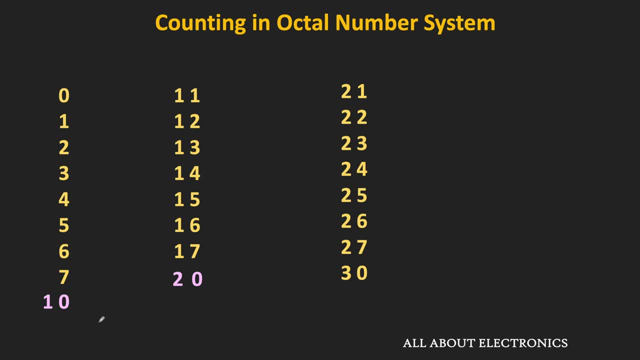 So that is how the counting is done in the octal number system, And here is the list of corresponding decimal numbers. That means the 8 in the decimal corresponds to 1: 0 in the octal number system. Likewise, the 24 in the decimal corresponds to 3: 0 in the octal number system. 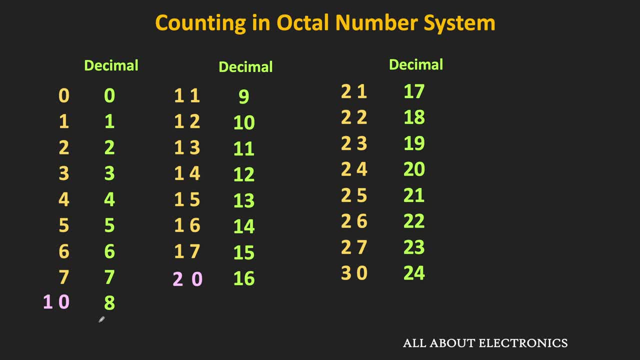 So later on we will see that, how to convert the octal number into the decimal equivalent number And vice versa, how we can convert this decimal number into the octal number. But first of all let's see how to convert this octal number into the binary equivalent. 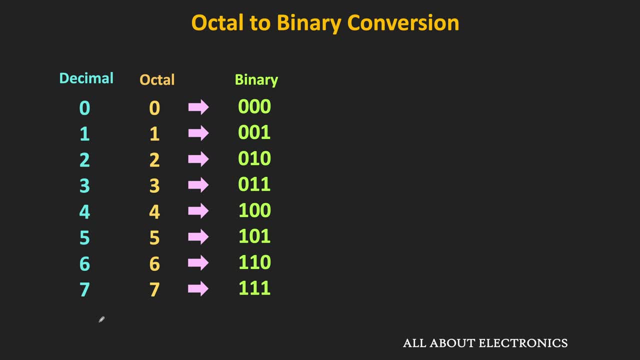 number. So here is the binary equivalent numbers corresponding to each octal digit. So to convert the octal number into the binary equivalent, we will replace each octal digit by the corresponding 3-bit binary number. So let's say we have an octal number 6573.. 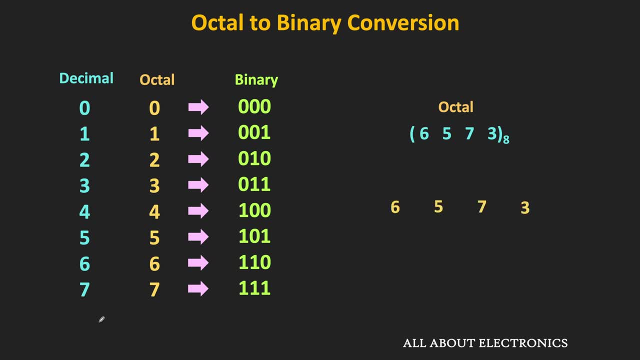 So for the octal to binary conversion, we will replace each octal digit by the corresponding 3-bit binary number. So here the binary equivalent of the 6 is equal to 110.. Likewise, the binary equivalent of the number 5 is equal to 101.. 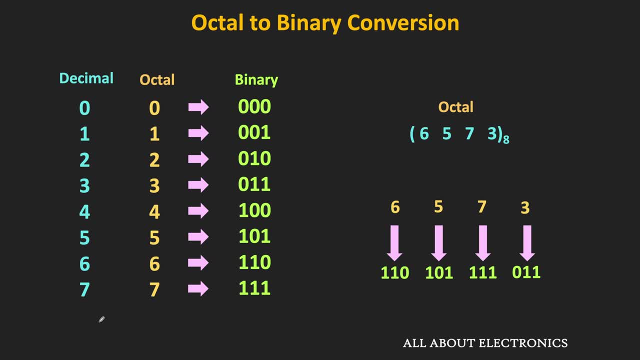 Similarly, we can replace this 7 by 111.. And likewise, these 3 can be replaced by 011.. So here is the binary equivalent of the 6.. So now, if we group all these binary numbers together, then this is the binary equivalent. 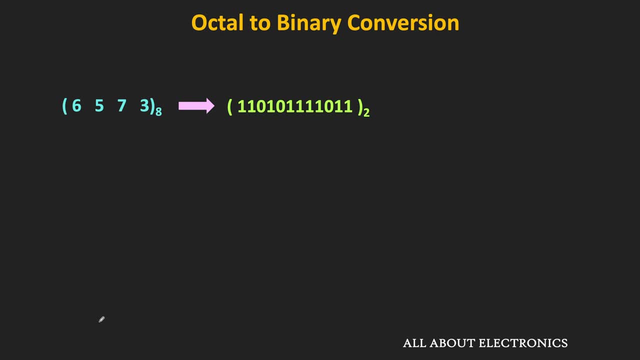 of the given octal number. So now let's take one more example, which also contains the fractional part. So first of all let's write down each octal digit, And now let's replace each digit by the equivalent 3-bit binary number. 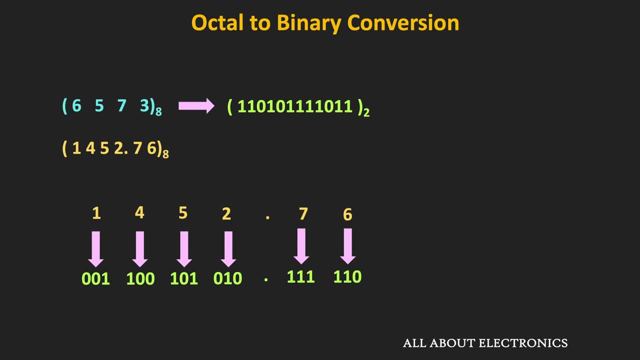 So here this 1 can be replaced by 001,, while the 4 can be replaced by 100.. Likewise, these 3 can be replaced by 100.. These 5 can be replaced by 101,, while the 2 can be replaced by 010.. 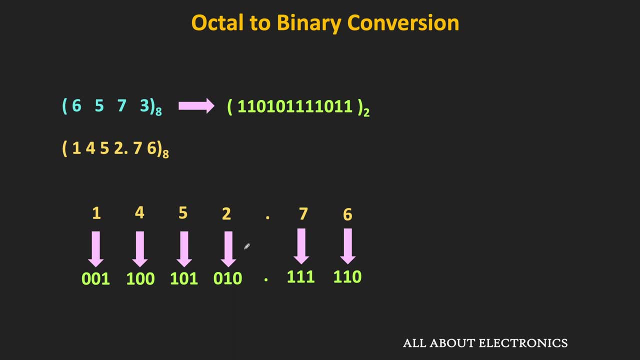 Then, after we will have this binary point, And after this binary point, these 7 can be replaced by 111, while the 6 can be replaced by 110.. So, while writing the overall binary equivalent number, these two zeros on the left can be. 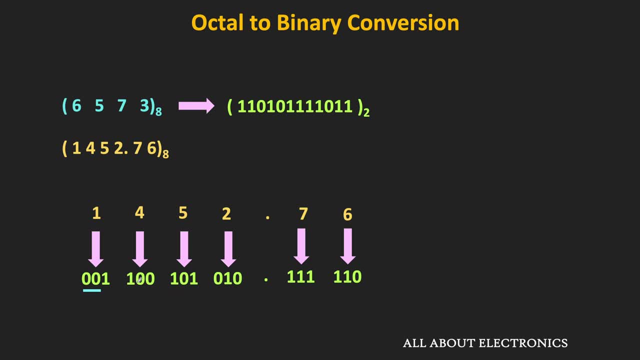 neglected Because these two zeros does not carry any value. Likewise, after this binary point, these rightmost zeros also carry any value. zero also does not carry any value. That means, while writing the overall binary equivalent number, this zero can also be neglected. That means this is the overall binary equivalent of the given. 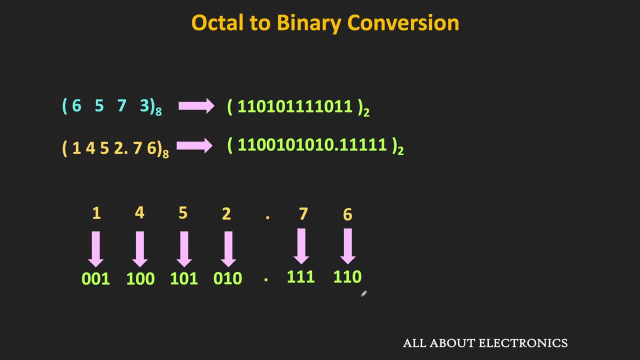 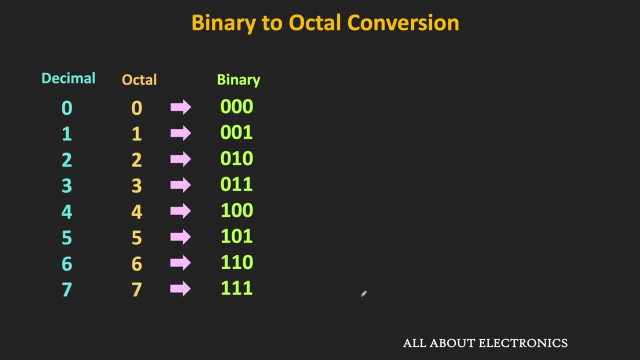 number. So that is how we can convert any octal number into the corresponding binary equivalent number. So, similarly, now let us see the binary to octal conversion. So for the binary to octal conversion, starting from the least significant bit, we will make the group of 3 binary digits. 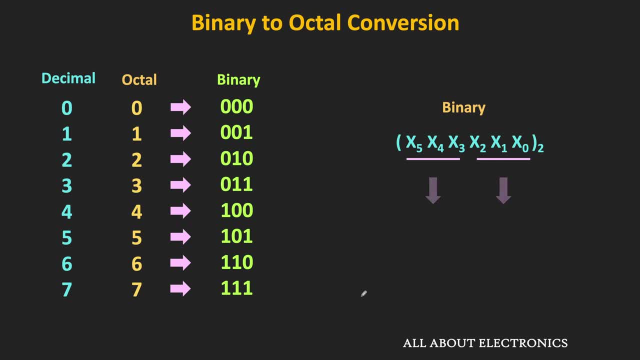 And then we will replace each group by the corresponding octal digit. So let's say we have a binary number- 100101. And we want to find the equivalent octal number. So first, starting from the LSB, let us make the group of 3 bits And then let us replace. 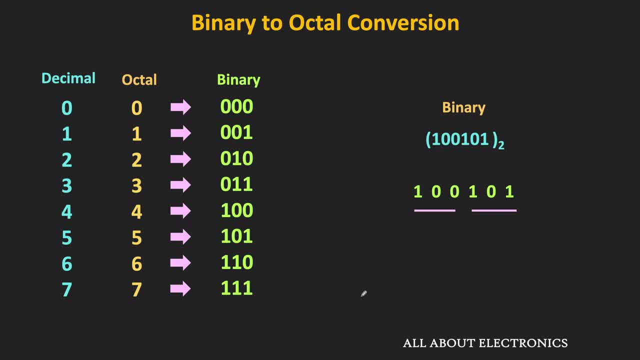 each group by the corresponding octal digit. So here this 100 corresponds to 4. And likewise this 101 corresponds to 5. That means, for the given binary number the equivalent octal number is equal to 45. So let us take one more example. 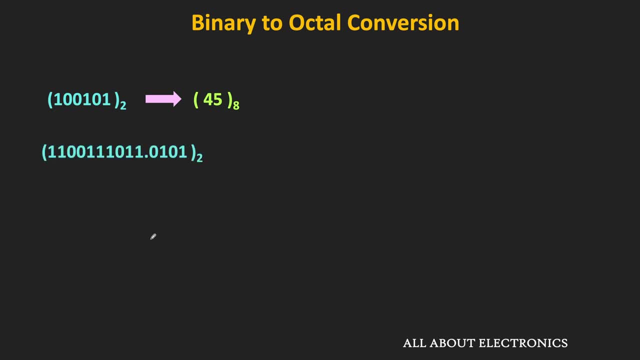 which also contains the fractional part. So let's say we want to find the equivalent octal number of the given binary number. So starting from this binary point, let us make the group of 3 bits both on the left and the right-hand side. 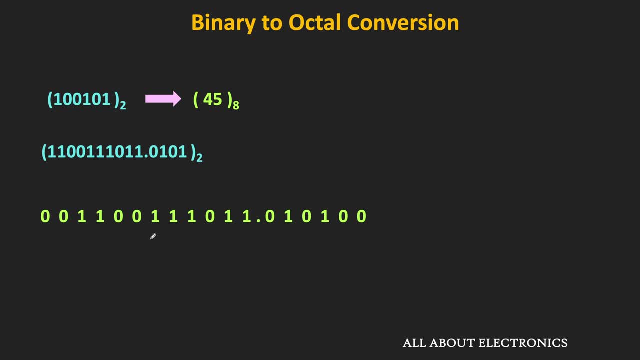 So on the left-hand side of this binary point the first group is 011.. Then the next group is 1111.. Likewise, the third group is 100 and the fourth group is 001.. So here to make a group of 3 bits, two more zeros are added over here, Similarly, after this binary. 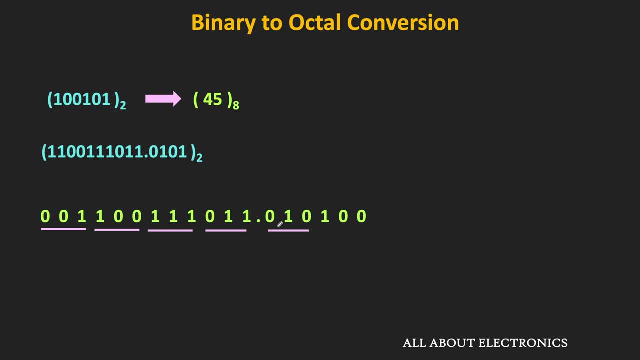 point. the first group is 010, while the second group is 100.. So over here also to make a group of 3 bits. two more zeros are added at the end. So now this 001 corresponds to 1 in the octal number. 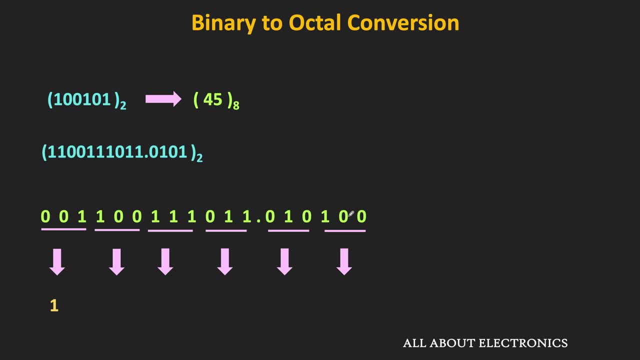 system. Likewise, this 100 corresponds to 4.. Similarly, this 111 corresponds to 7, while this 011 corresponds to 3.. Similarly, after this octal point, this 010 corresponds to 2, while the 100. 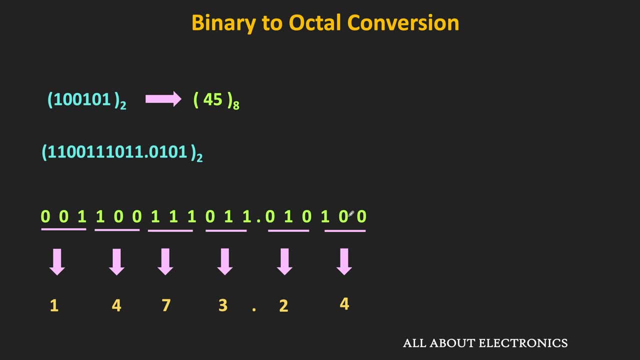 corresponds to 4.. So here to make a group of 3 bits, two more zeros are added over here. So now That means for the given binary number the equivalent octal number is equal to 1473.24.. So in this way we can convert any binary number into the equivalent octal number. 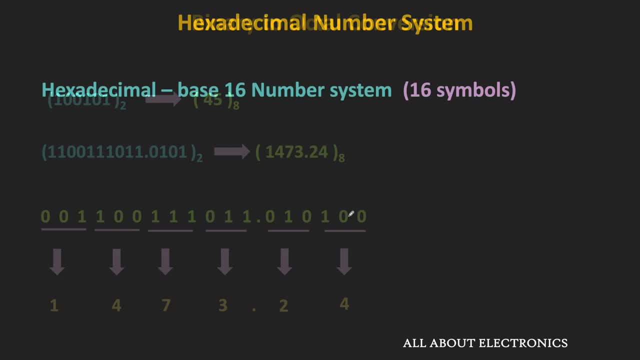 Alright, so similarly, now let's understand about this hexadecimal number system. So, as I said earlier, this hexadecimal number system is a base 16 number system And it consists of total 16 symbols. And here is the list of all 16 symbols. 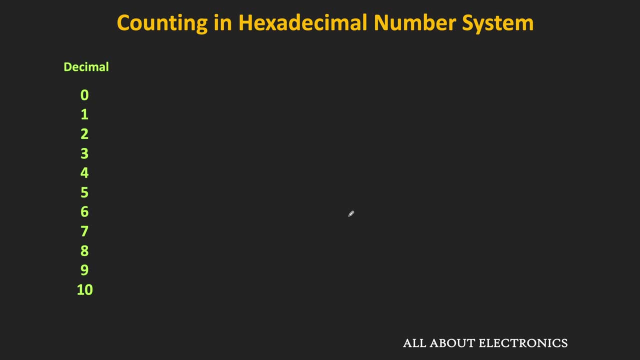 So if we compare this system with the decimal number system, then the 0 to 9 in the hexadecimal number system is same as the decimal number system, But the 10 in the decimal corresponds to A in the hexadecimal number system. Likewise, this 11 in the decimal number system corresponds to B in this hexadecimal number. 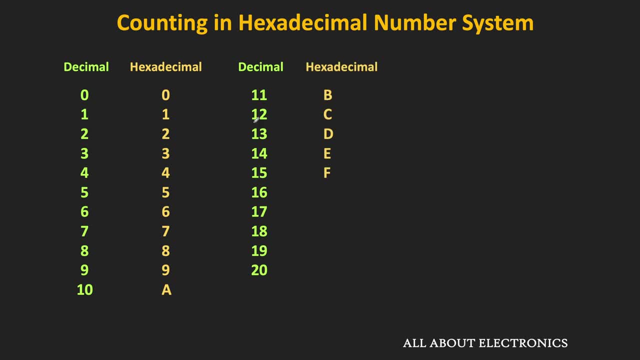 system. And likewise this 12 corresponds to C And this 13 corresponds to D. Similarly, These 14 and 15 in the decimal number system corresponds to E and F in this hexadecimal number system. So that is all the 16 symbols of this hexadecimal number system. 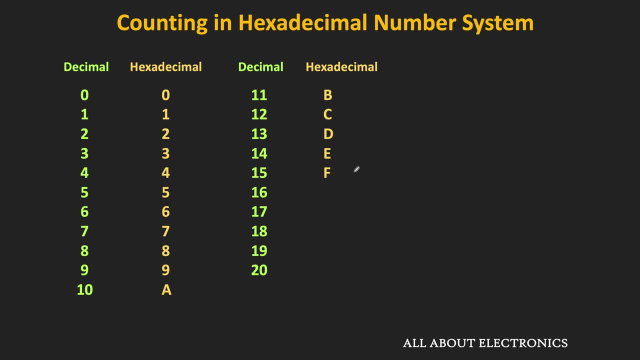 So if we want to count further, then we will reset that column to the 0, and we will increment the next column by the 1. That means after the F the next number in the counting is equal to 10.. That means the 16 in the decimal number system corresponds to 10 in this hexadecimal number. 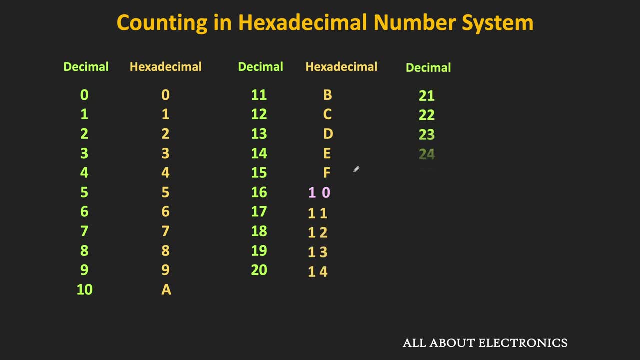 system And if we continue the counting then we can go up to 1F. So once again in this rightmost column we have used all the symbols of that particular number system. That means after that we can reset that column to the 0, and we can increment the next column. 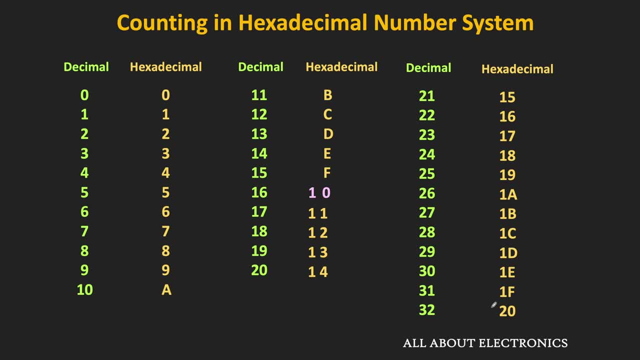 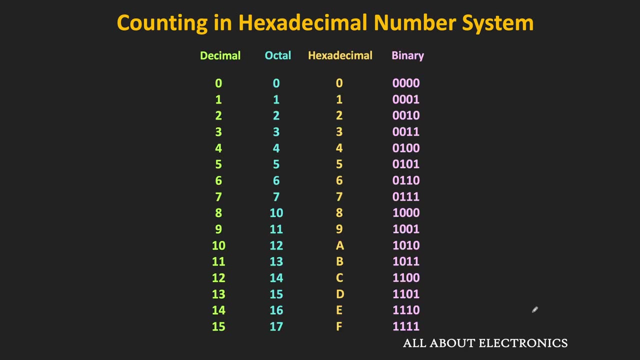 by 1.. That means after 1F the next number will be equal to 20.. And then, after, the counting will go on. So that is how we can count in this hexadecimal number system. And here is the list of numbers 0 to 15 in the octal hexadecimal and the binary number. 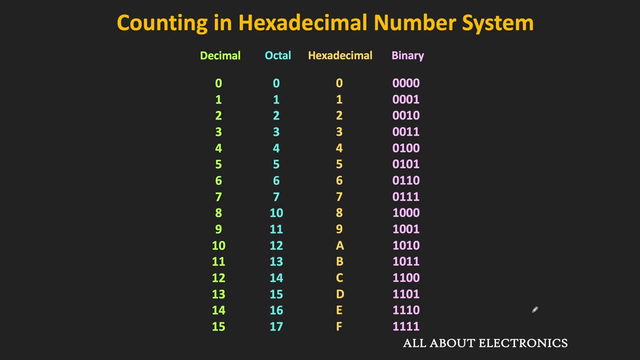 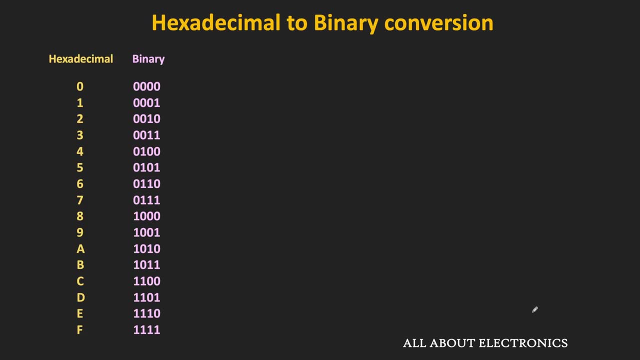 system. So now let's see how to convert any hexadecimal number into the corresponding binary equivalent number. So for this hexadecimal to binary conversion, we will replace each hexadecimal digit by the equivalent 4-bit binary number. So let's say we want to convert this hexadecimal number into the corresponding binary number. 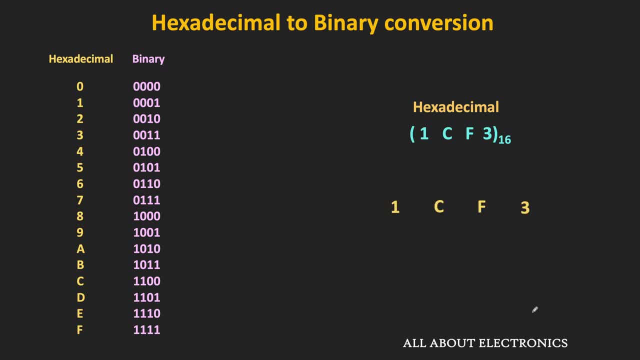 So first of all, let's convert this hexadecimal to the corresponding binary number. First of all, we will replace each hexadecimal digit by the corresponding 4-bit binary number. So here this 1 corresponds to 0001,, while this c corresponds to 1100.. 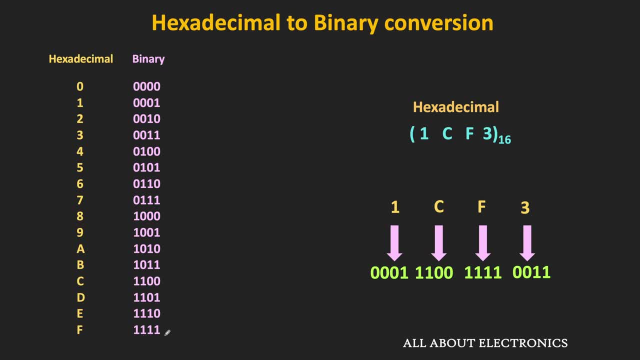 Likewise, this f corresponds to 1111, while this 3 corresponds to 0011.. So if we combine all these binary groups, then this is the binary equivalent number of the given hex number. So let's take one more example which also includes the binary equivalent number. 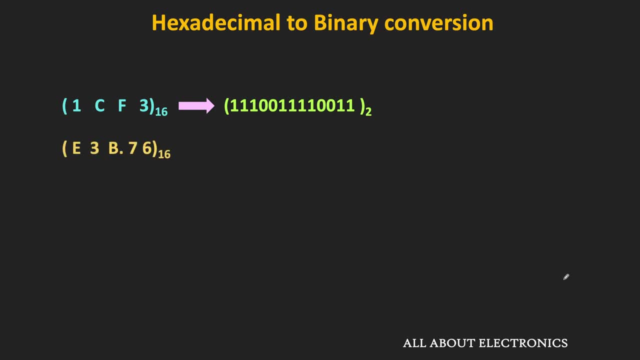 So let's take one more example which also includes the binary equivalent number of the given hex number. So let's take one more example which also includes the binary equivalent number of the given hex number. So let's take one more example which also includes the binary equivalent number of the. 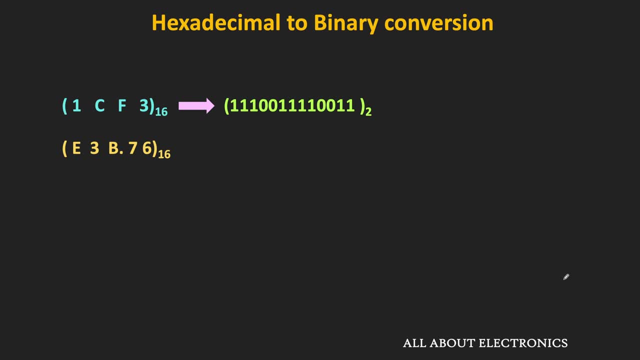 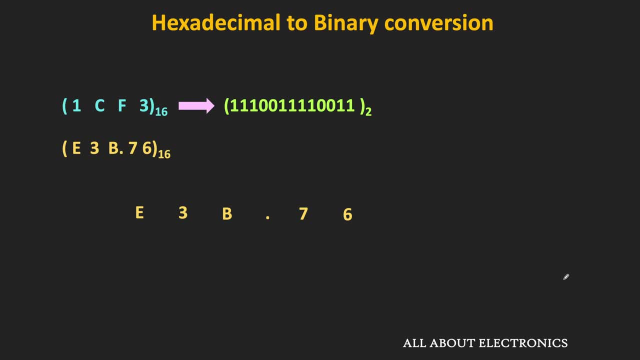 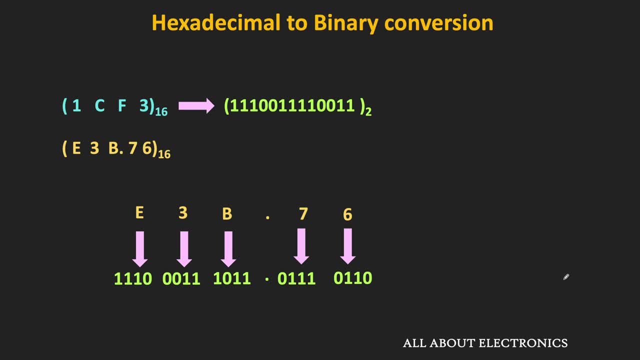 given hex number. So let's take one more example, which also includes the binary equivalent number of the digits. And if we combine all these binary groups, then this is the binary equivalent number of the given hex number. So that is how we can convert any hexadecimal number into the binary equivalent number. 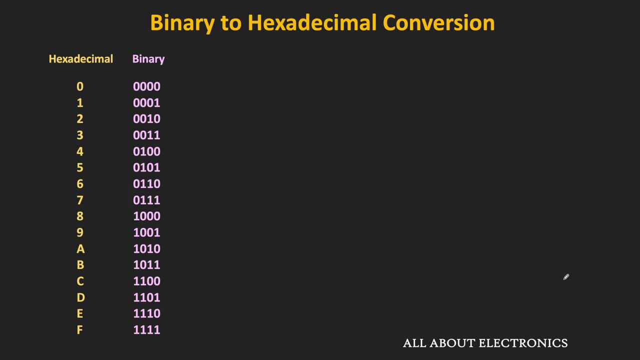 So similarly, now let's see the binary to hexadecimal conversion. So for the binary to hexadecimal conversion, starting from the LSB, we will make the group of 4 bits And then we will replace each group by the corresponding hex digit. So let's say we have this binary number and we want to convert it into the equivalent. 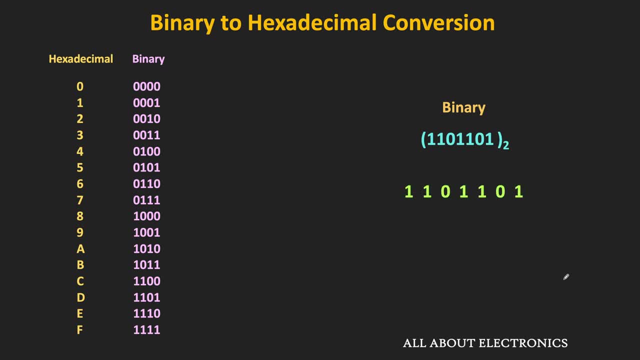 hexadecimal number. So first of all, starting from the LSB, let's make the group of 4 bits. So here the one group is 11,, 0,, 1.. And to make the second group, here we will add one more, 0. 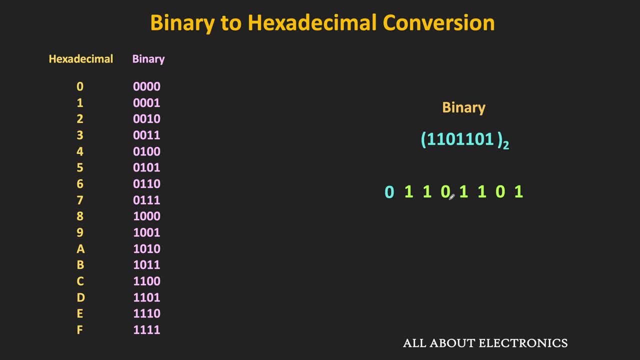 That means the second group is 01, 10.. So this 01, 10 corresponds to 6,, while this 11, 0, 1 corresponds to d. That means for the given binary number the equivalent hex number is equal to 6d. 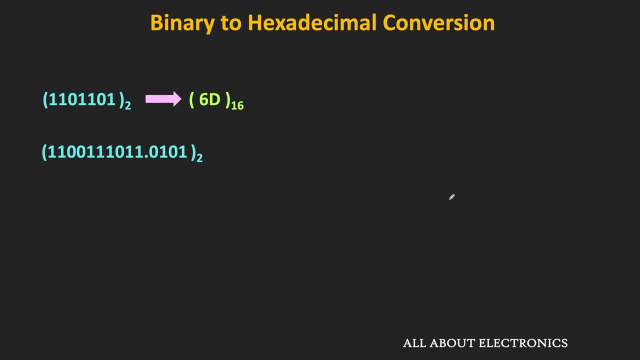 So let's take one more example. So let's say we want to find the equivalent hex number of the given binary number. So first of all, starting from the binary point, let's make the group of 4 on both sides, So on the left-hand side. 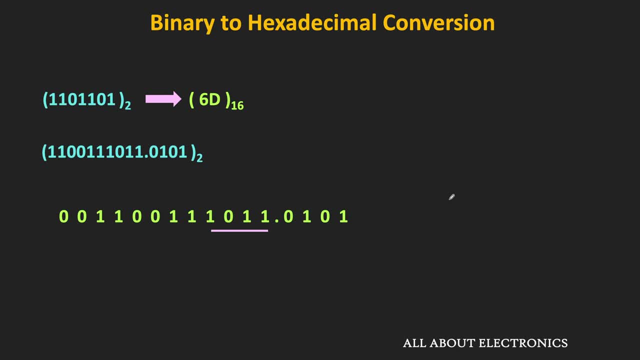 the first group is 10, 1, 1,, then the next group is 00, 1, 1.. Likewise, the third group is also 00, 1, 1.. Similarly, on the right-hand side of this binary point, the 4-bit group is 0, 1, 0, 1.. 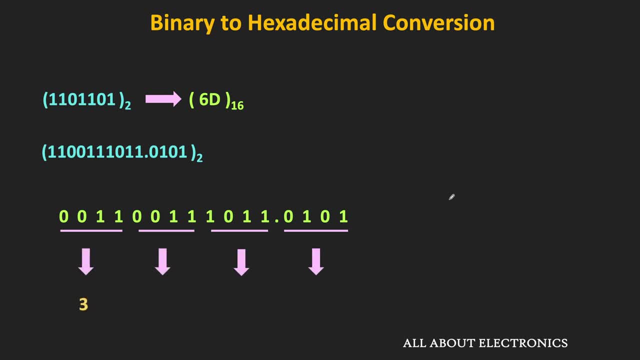 So now this 00, 1, 1 corresponds to 3,, while this 00, 1, 1 also corresponds to 3.. Then this 10, 1, 1 corresponds to b And this 0, 1, 0, 1 corresponds to 5.. 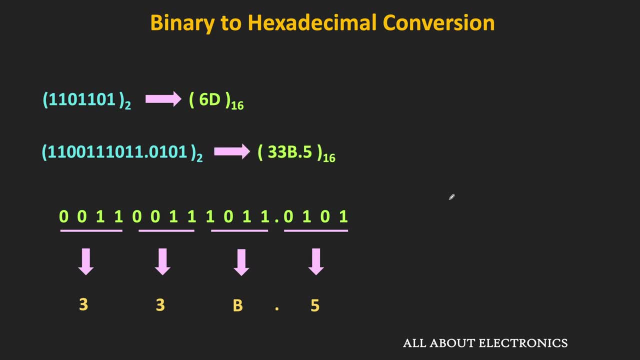 That means for the given binary number, the equivalent hex number is equal to 33b.5.. So that is how we can convert any binary number into the equivalent hexadecimal number. Alright, so now let's see how to convert any octal or the hexadecimal number into the 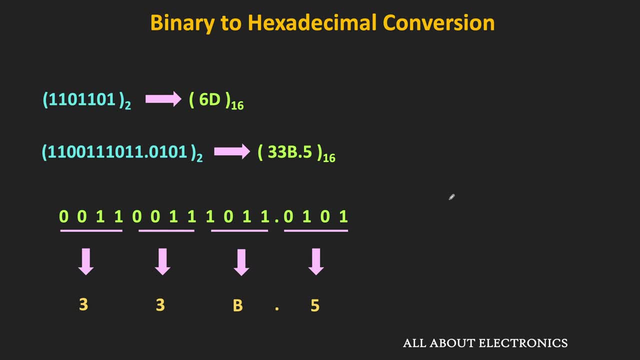 decimal equivalent number. And first let's see the octal to decimal conversion. So in the earlier videos we have seen that if we have any number we have to convert it into a decimal equivalent In the base-b-number system. then this is how we can convert it into the equivalent. 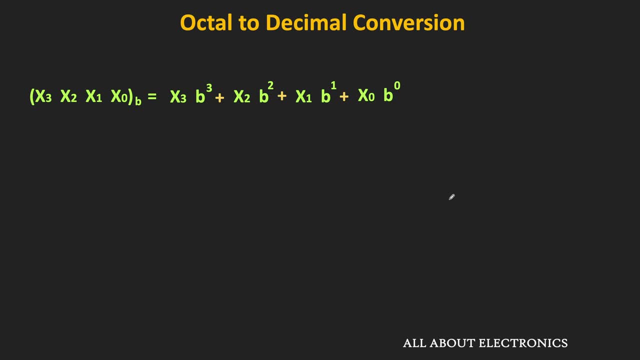 decimal number. So here this b corresponds to the base of that particular number system. So suppose if we have a number in the octal number system, then this is how it can be converted into the decimal number. So here this least significant digit has the weightage of 1.. 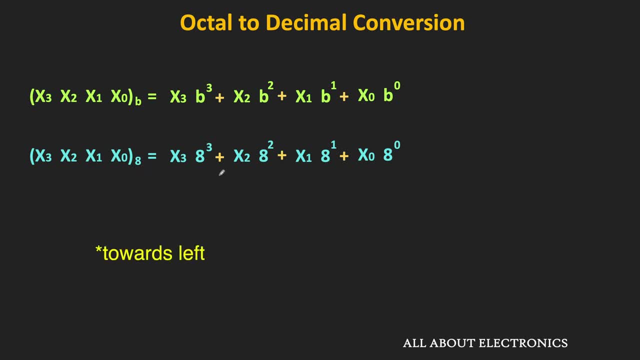 And as we move towards the right then the weightage of each digit will increase by the factor of 8.. So if we just add all these terms then we will get the equivalent decimal number. So let's say we have some octal number, 4126, and we want to find its equivalent decimal. 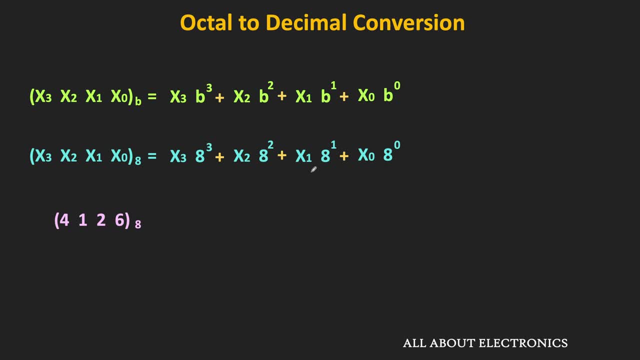 number. So for that let us write down each digit with their corresponding weight and then let us add them all. So here this 6 into 8 to the power 0 is equal to 6.. Then this 2 times 8 to the power 1 is equal to 16.. 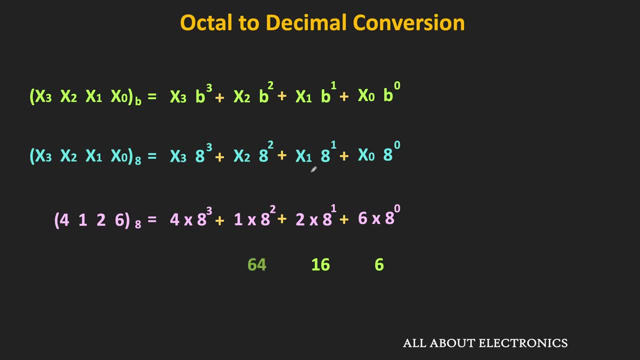 Likewise, this 1 times 8 to the power 2 is 64. While this 4 times 8 to the power 3 is equal to 2048.. So if we do the summation of all these numbers, then it is equal 2, 1,, 3, 4.. 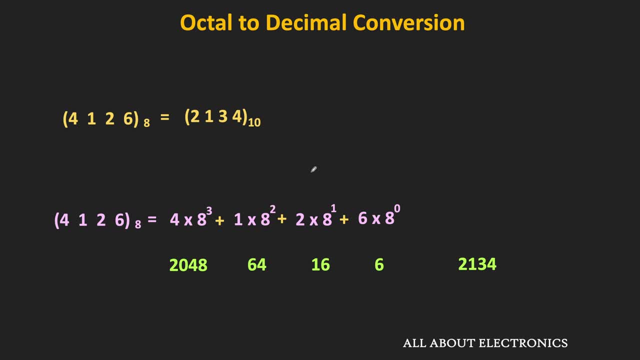 That means the decimal equivalent of the given octal number is equal to 2134.. Now suppose we have a fractional part. then for the fractional part also the procedure will remain the same. So after that octal point, As we move towards 3.. 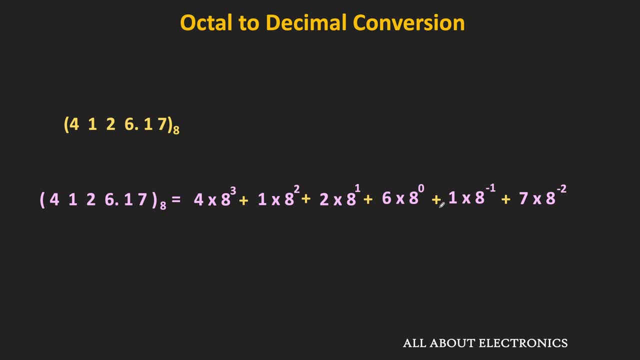 right, then the weightage of each digit will reduce by the factor of 8.. So here the initial 4 digits are same And, as we have seen, their summation is equal to 2134.. So after this octal point, this 1 by 8 corresponds to 0.125,, while this 7 times 8 to the power. 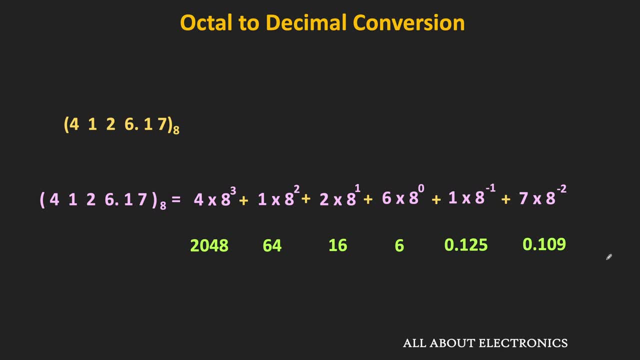 minus 2 corresponds to 0.109.. So if we add all these terms, then their summation is equal to 2134.234.. So that is the decimal equivalent of the given octal number. So in this way we can perform the octal to decimal conversion. 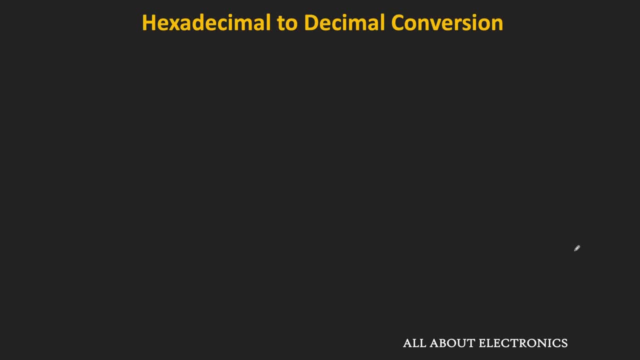 And similarly we can also do the hexadecimal to the decimal conversion, But in this case the weightage of each digit will increase or reduce by the factor of 16.. So let's say we want to find the decimal equivalent of the given hex number. 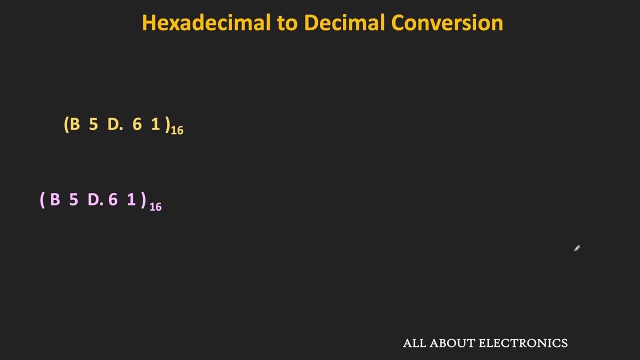 So, starting from the hexadecimal point, as we move towards the left, then the weightage of each digit will increase by the factor of 16.. And as we move towards the right from this hexadecimal point, then the weightage of each digit will reduce by the factor of 16.. 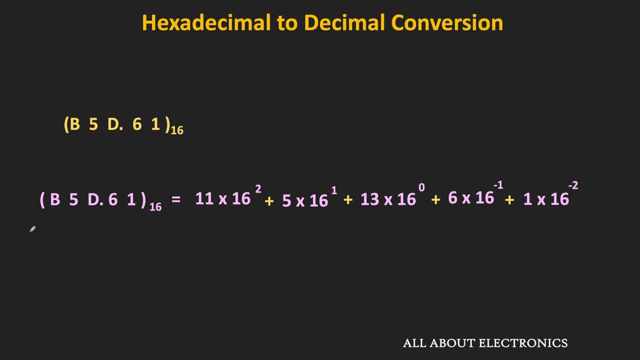 So here this D corresponds to 13,, while this B corresponds to 11.. So if we add all these terms, then their summation is equal to 2909.374.. So that's it. So that is the decimal equivalent of the given hex number. 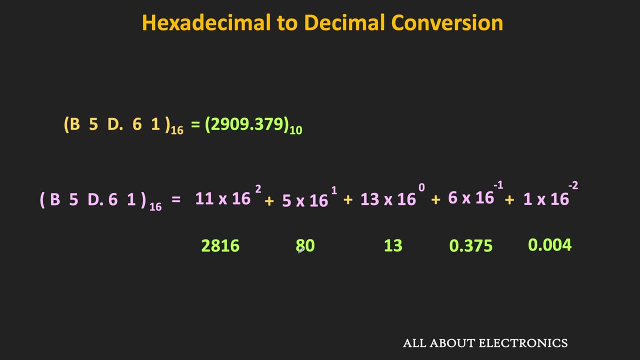 So in this way we can convert any hexadecimal number into the decimal equivalent number. Alright, so so far we understood that how to find the decimal equivalent of the given octal or the hexadecimal number. So similarly, now let's see, suppose we have been given some decimal number. then how to? 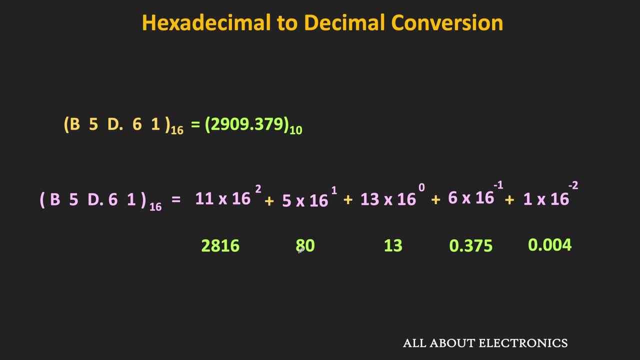 convert it into the equivalent octal or the hexadecimal number. And first of all let's see this decimal too. So let's say we want to convert this decimal to octal conversion. So during the decimal to binary conversion, we have seen that by successfully dividing 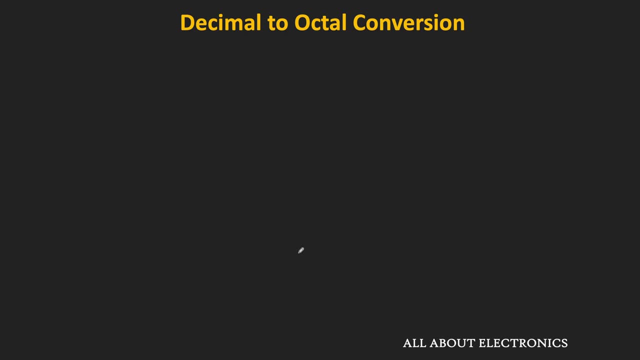 this decimal number by the 2, we can get the binary equivalent number. So similarly for the decimal to octal conversion we will successfully divide the decimal number by the 8.. So let's say we want to convert this decimal number, 120, into the octal number. 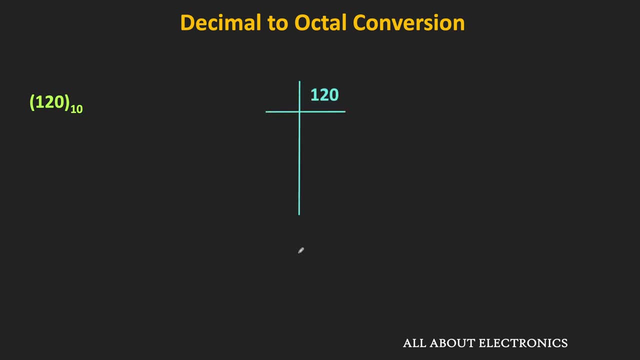 So for that, let's divide this number by the 8.. So after the first division, So after the first division, The quotient will be equal to 15, while the remainder is equal to 0. Similarly, when the second time we divide this number by the 8, then the quotient is: 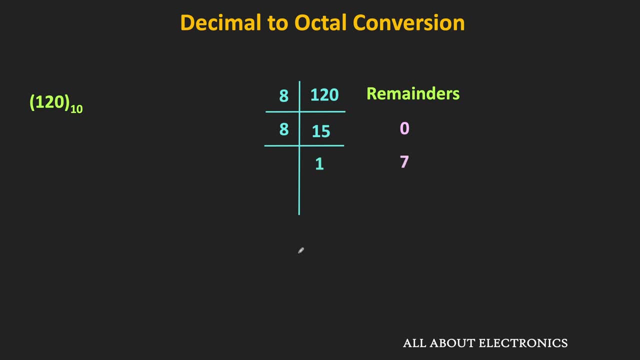 equal to 1 and the remainder is equal to 7.. Now, once again, if we try to divide this number by 8, then we cannot divide it. That means the quotient is equal to 0 and the remainder is equal to 1.. 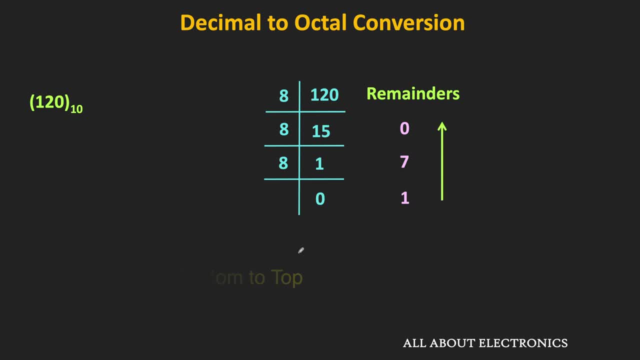 And if we write down all these remainders from top to bottom, then we will get our octal equivalent of the given octal, Given decimal number. That is equal to 170.. Now suppose the decimal number also contains some fractional part. then we will treat the 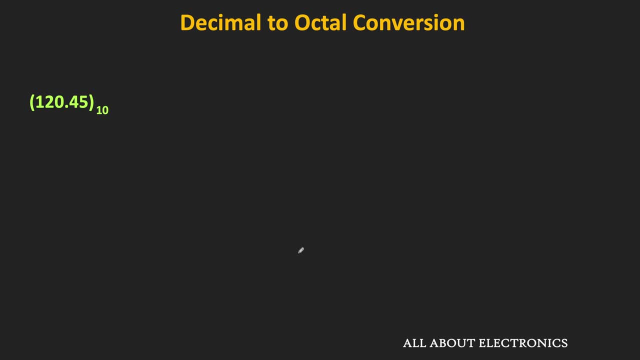 integer and the fractional parts separately. So for the integer part, by following the same procedure, we can find the equivalent octal number, While for this decimal fractional part, by successfully multiplying it by the factor of 8, we can find the equivalent octal number. 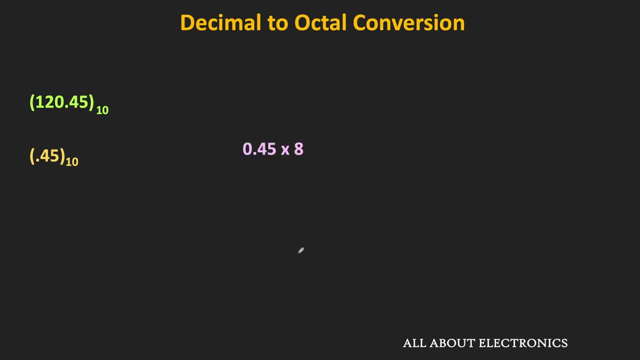 So first time, if we multiply this 0.5 by 8. Then, after multiplication, the number is equal to 3.6.. So from this 3.6, this 3 is the integer part, while the 0.6 is the fractional part. 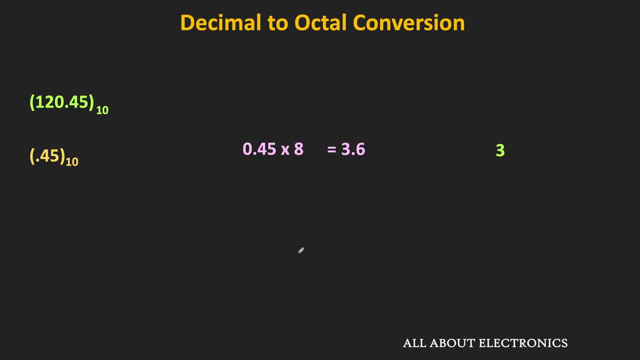 So let us write down this integer part separately. So once again, if we multiply this 0.6 by the 8, then after the multiplication the number is equal to 4.8.. So once again, let us write down this 4 separately. 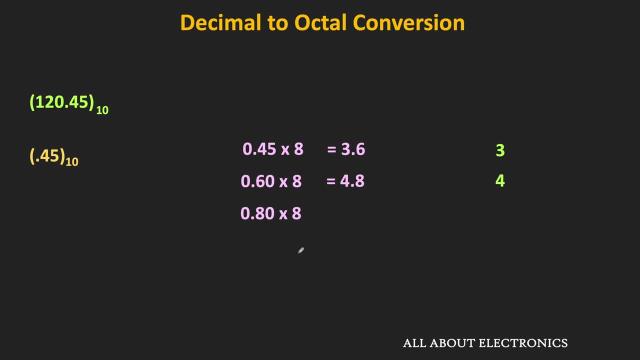 And let us multiply this fractional part by 8.. So if we follow the same procedure for couple of times, then these are the integer parts. So let's write down these integer parts from top to bottom, And in fact it is the equivalent octal number of the 0.45.. 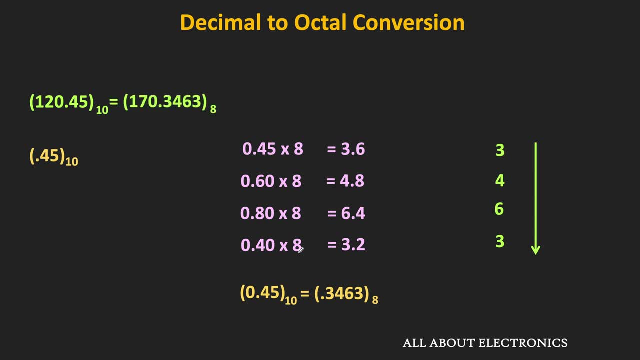 That means, for the given decimal number, the equivalent octal number is equal to 170.3463.. So that is how we can convert any decimal number into the equivalent octal number. Alright, So similarly, now let's see the decimal to hexadecimal conversion. 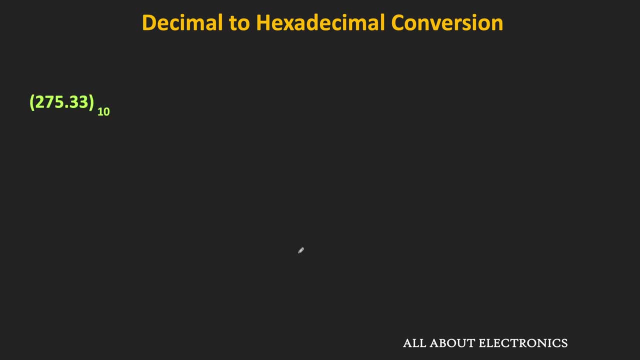 So let's say we want to convert this decimal number into the equivalent hex number. So, as I said, we will consider the integer and the fractional parts separately. So for the integer part, by successfully dividing this number by 16, we can find the equivalent. 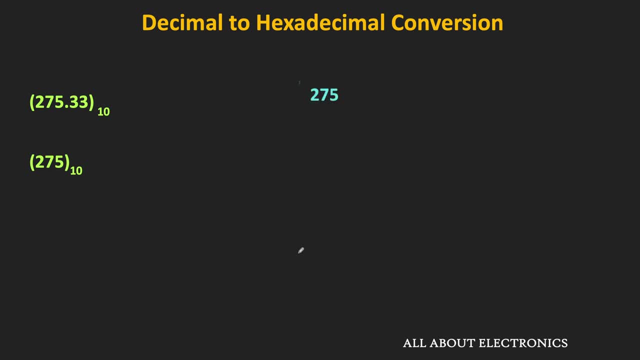 hex number. That means, if we divide this 275 by 16,, then the quotient is equal to 17 and the remainder is equal to 16.. Now the increment is 16.. If we divide it by 16,, then the equivalent is equal to 3.. 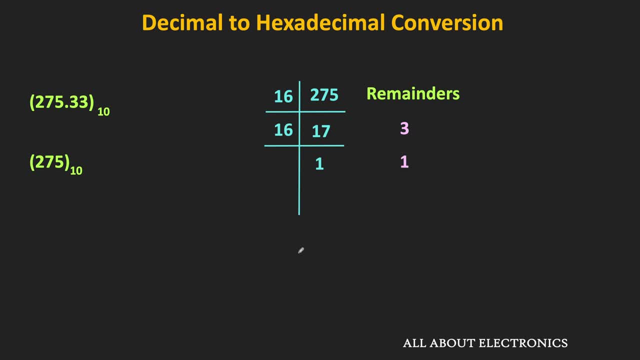 If we write down these remainders from bottom to epi, that's 1,, 1,, 3, and we shit here it's 113.. So once again, if we divide it by the 16, then the quotient is 1, and the remainder 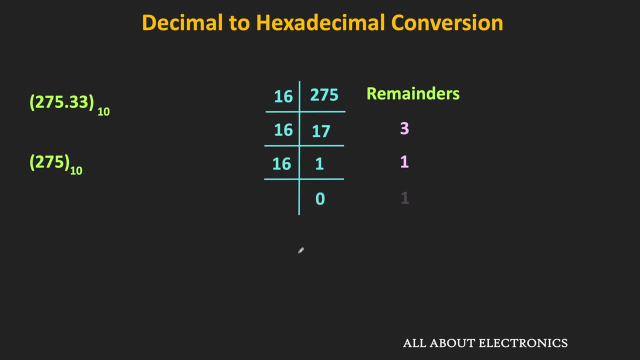 is also 1.. Now if we try to divide this 1 by 16,, then we cannot divide it. That means now the quotient is 0, while the remainder is equal to 1. And if we write down these remainders from bottom to top, then we will get our equivalent. 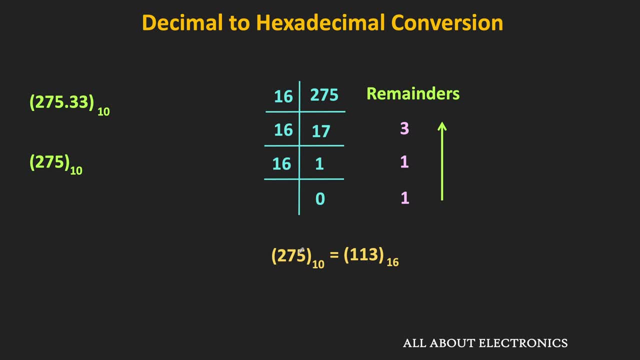 hex number That is equal to 113.. number. Similarly, let's find out the hex number for the fractional part. So for this fractional part, we will successfully multiply this fractional part by 16.. So for the first time when we multiply it by 16, then after the multiplication, the 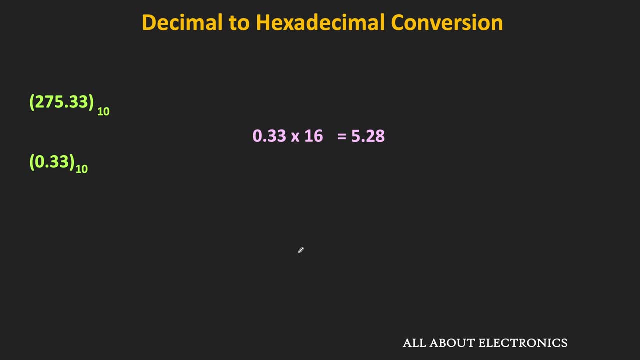 number is equal to 5.28.. So let's write down this integer part separately And let's multiply this fractional part once again. So after the multiplication, the number is equal to 4.48.. So once again, let's write down this integer part separately. 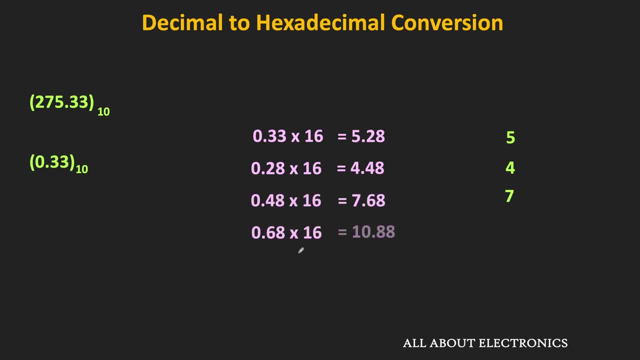 And if we follow the same procedure for couple of times, then these are the integer numbers, And here this 10 corresponds to a in the hexadecimal number system. So if we write down all these integers from top to bottom, then we will get our equivalent. 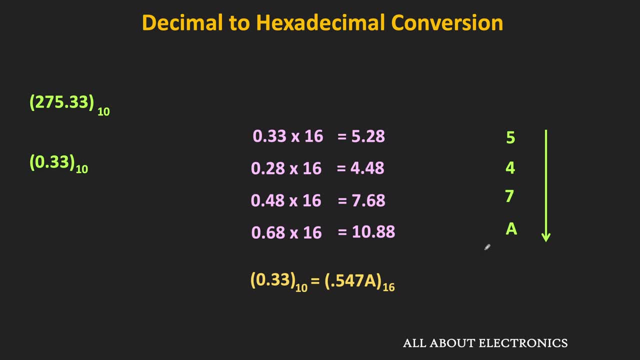 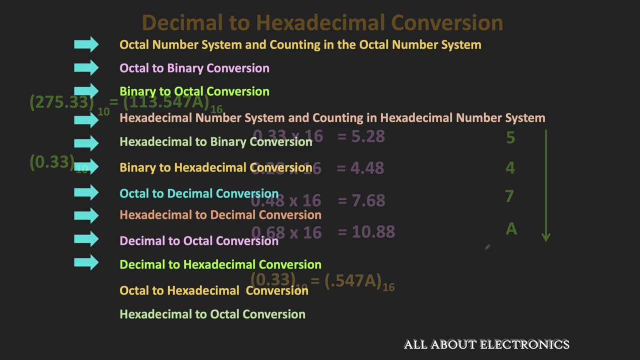 hex number That is equal to 0.547a. That means the equivalent hexadecimal number for the given decimal number is equal to 113.547a. So in this way we can convert any decimal number into the equivalent hex number. Now, so far we have seen the following conversions: 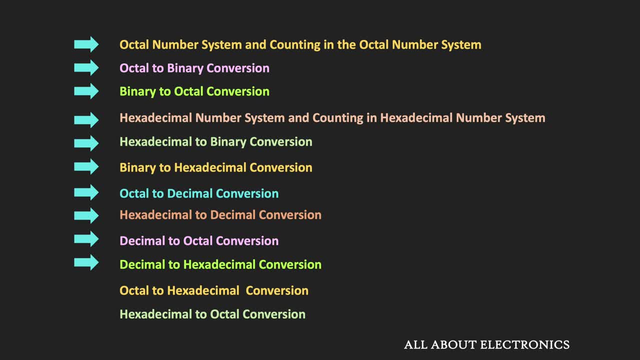 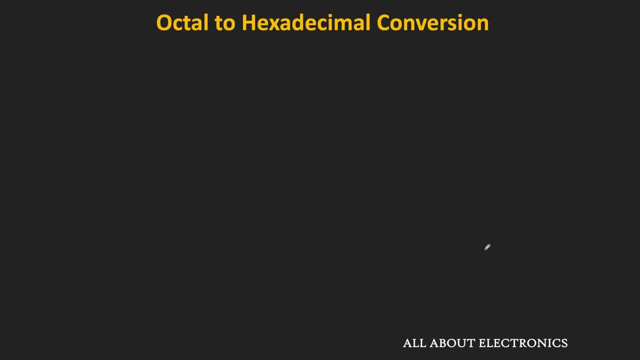 So the only thing which remains is the octal to hex and the hex to octal conversion. And first let's see how to convert any octal number into the equivalent hex number. So it is very simple. So first convert the octal number into the equivalent binary number and then convert. 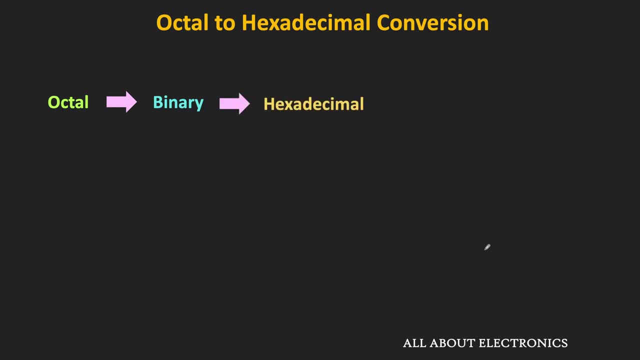 this binary number into the equivalent hex number. So let's take one example. So let's say we want to convert this octal number into the equivalent hex number. So first of all we will find its equivalent binary number And for that we will replace each octal digit by the equivalent 3-bit binary number. 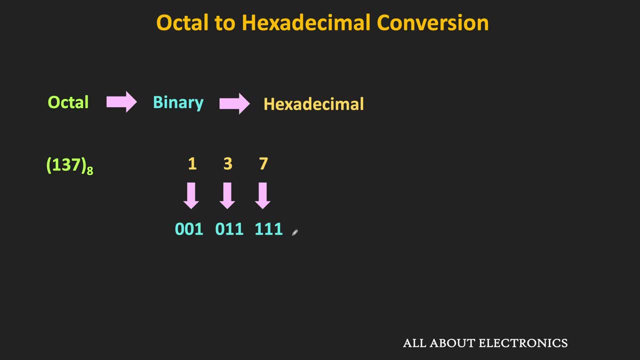 So these are the equivalent binary numbers for the given octal digits. So if we combine all these binary groups, then this is the equivalent binary number of the given octal number. Now for the binary to hex conversion. starting from the LSB, we will make a group of 4 bits. 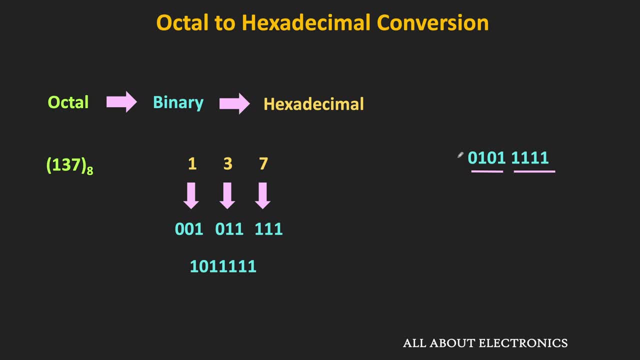 So here, just to make a group of 4, one more zero is added over here, And now let us replace each group by the corresponding hex digit. So these 0101 corresponds to 5.. While these 1111 corresponds to f. 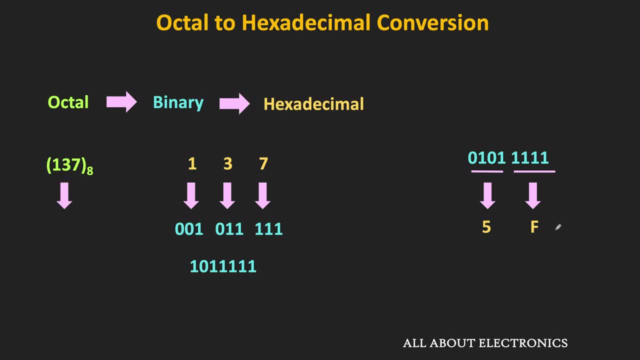 That means for the given octal number, the equivalent hex number is equal to 5f. So this is fine. Ok, So that is how we can perform the octal to hexadecimal conversion, And similarly we can also convert any hex number into the equivalent octal number. 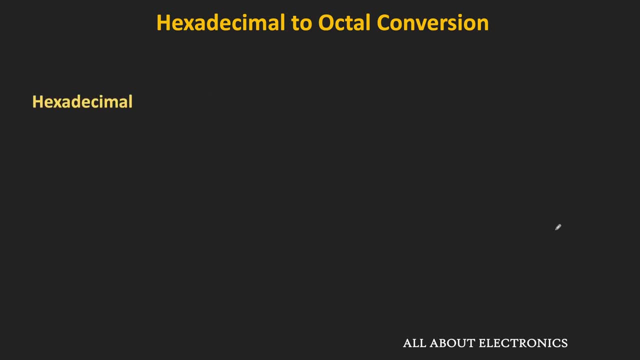 So for that, first of all we will convert the hex number into the equivalent binary number And then we will convert this binary number into the equivalent octal number. So let's take one example. So let's say we want to convert this hex number into the equivalent octal number. 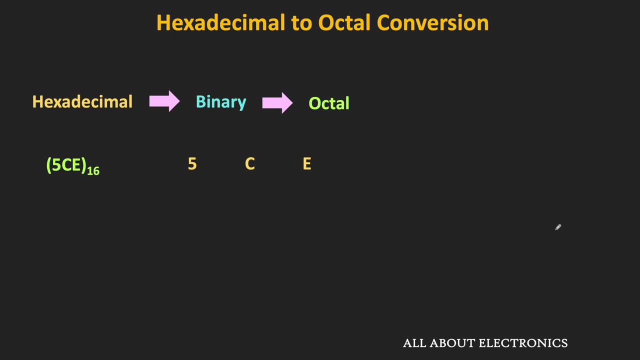 So first of all let's convert this hex number into the binary number, And for that we will replace each hex digit with the corresponding 4-bit binary number. So if we combine all these binary groups, then this is the equivalent binary number. 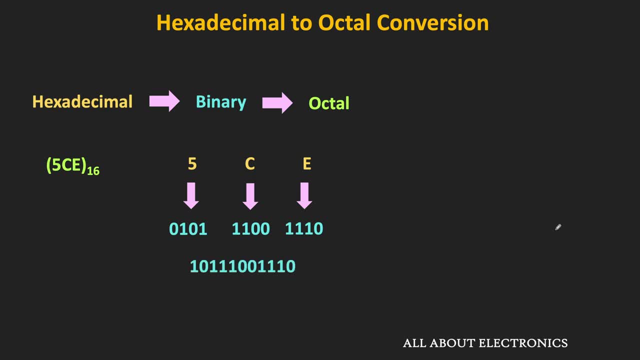 of the given hex number. Now to perform the binary to octal conversion, starting from the LSB, let's make the group of 3 bits And let's replace each group by the corresponding octal digit. That means for the given hex number. we will convert this hex number into the equivalent.